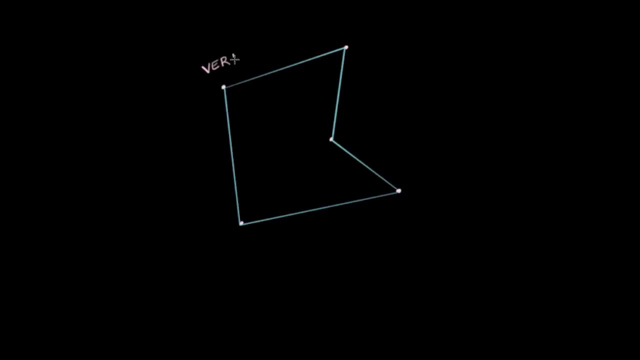 So a corner is also called a vertex, v-r-t-e-x. a vertex. Now that's just a very fancy sounding name for corner. so you can say corner if you want to, but if somebody else is vertex, now you know what they mean. they just mean the corner. Now you can see that this is a vertex. this is also a vertex. this. 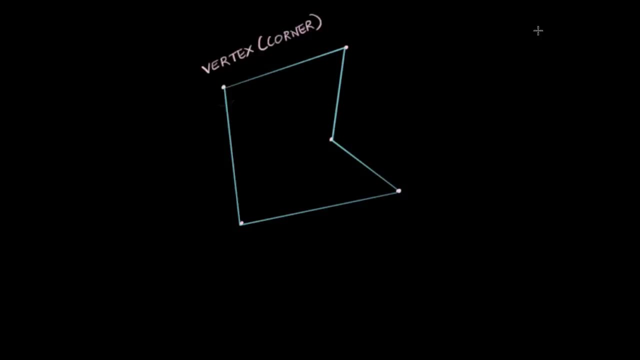 is also one, but if I want to talk about this one specially, then it's good to give it a name, and that's why we always give names, so that it's easy to talk about it. So I'm going to name this one a, this one b, then c, d. 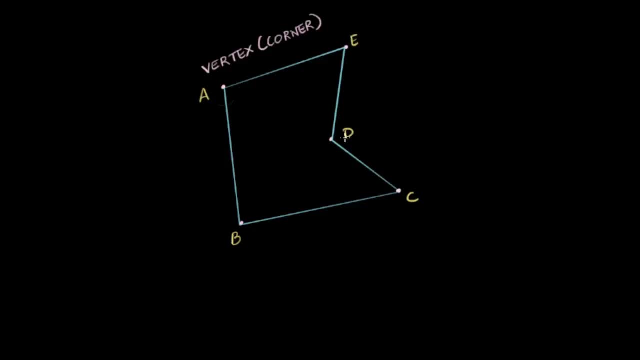 and e. Now, if I do this now, I can say I'm talking about the vertex d and you know exactly that I'm talking about this corner over here. Now another question can be: how do I refer to this polygon? Is there a way I can name this entire polygon? And one way to do that is to 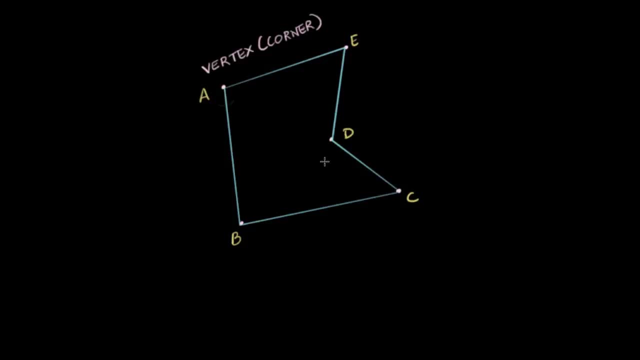 actually name it using its vertices. So I'm going to say: this is the polygon that goes from a to b to c, to d to e and then back. We know it has to go back because otherwise it won't be closed. So I can just say: a, b, c, d, e is this polygon. and there are many ways to name it. You can say: 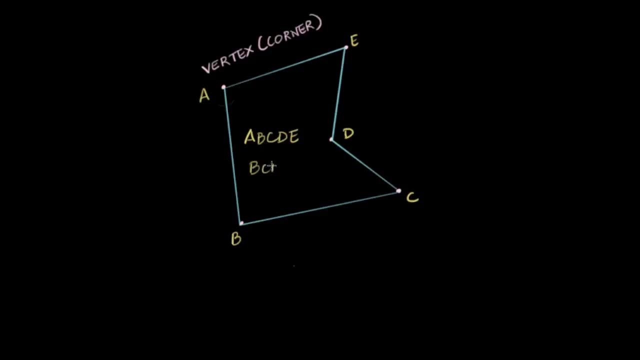 it's b, c, d e, a and that will also be fine. b c, d, e a. You can even go in the other direction. You can say: you know what this is. d, c, b, a e. d c, b, a e. That's also a valid way to a correct. 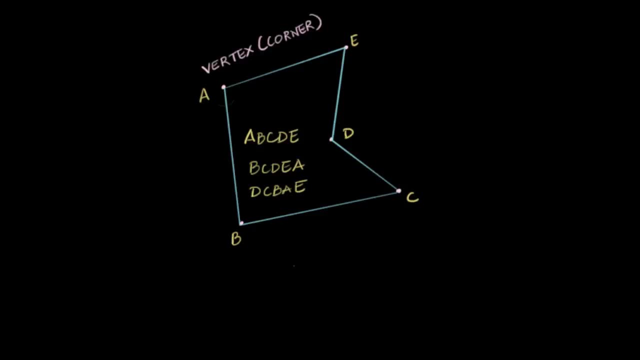 way to name this polygon. But if you do something like um, let me try this like d a, b, c, e. Let's say you say that d a, b, c, e. That's not this polygon, right, d and a are not even connected. 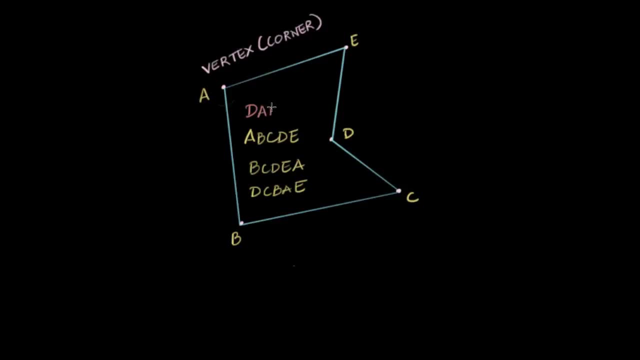 So when you say d a, b, c e, that's not correct. d a, b, c e, Then that's not correct. You're not really going in the order of this polygon. So I'm going to take away all of these other ones, because now 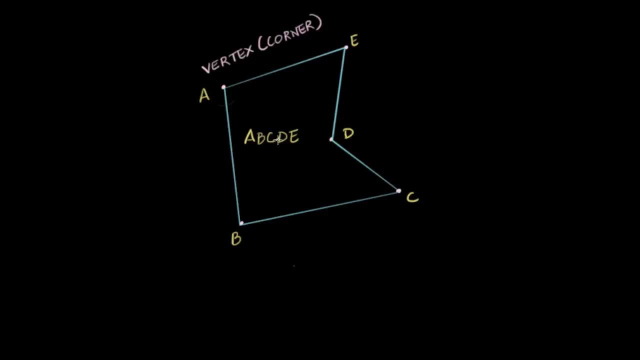 you know that order does matter. I'm just going to keep a b c d here, a b c d e over here as a way to name this polygon. You can also see, now that there is a line segment, that 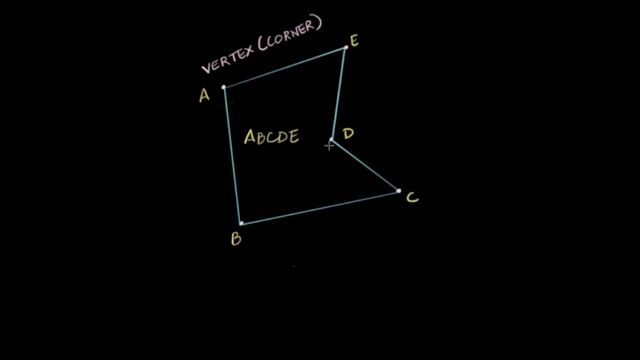 connects this vertex e to this vertex d, And there's another line segment that connects d to c. So there are these line segments And what do we call those? We call them sides of this polygon, And this might be familiar to you a little bit, because if I take something like a square, 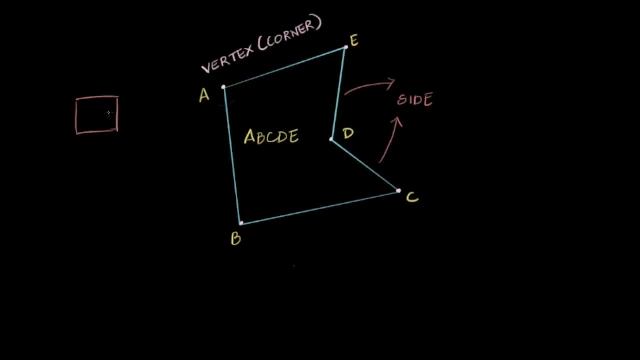 you know that if, if I just have a square here, even though this doesn't look too much, it does look like a square. So if I take a square and I say this is the side of a square, So that's just not true for a square or a rectangle. 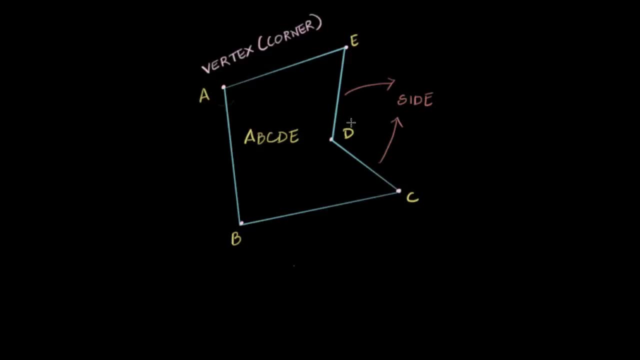 It's true for any polygon. All of them have these things called sides. But now again, this is a side, This is also a side. How do I differentiate between them? How do I tell I'm talking about this side? Now, one way to do that is to say: hey, I'm talking about the side that connects e and d. 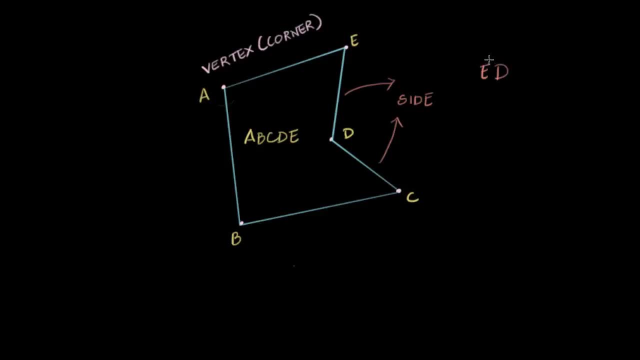 So how we write that is that I take I write e and d and I say and I put a line on top And the way I read it will be: it's the line segment that connects the points e and d. I can write the same thing as d, e. 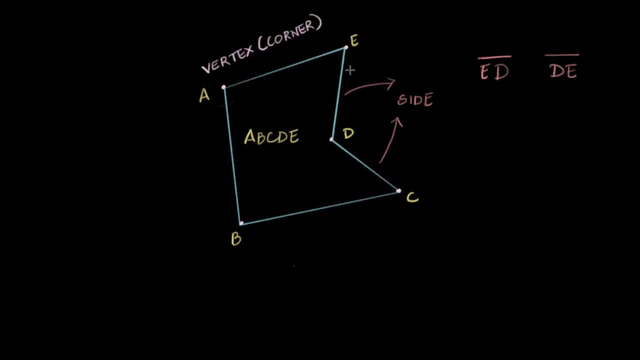 It won't make a difference. The order here does not matter. The line segment that connects d and e is the same line segment that connects e and d. So going by this, you can see that e- d is a side, e d with a line on top is a side, d? c is a side. So this is my side- d? c. So d? c is a side. 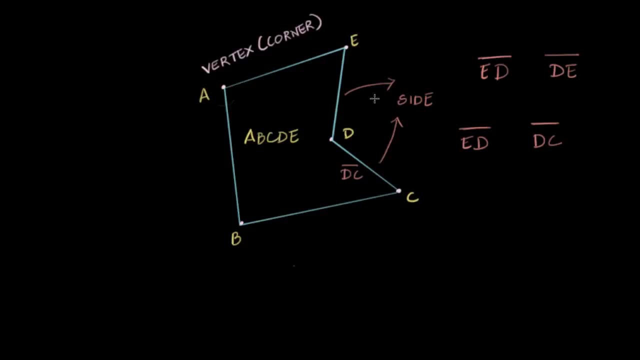 b, c is also a side. But before we go there, notice that e, d and d? c have something in common. And what is that? It's this vertex: d, So e, d and d? c share this vertex. So whenever that happens, when two sides 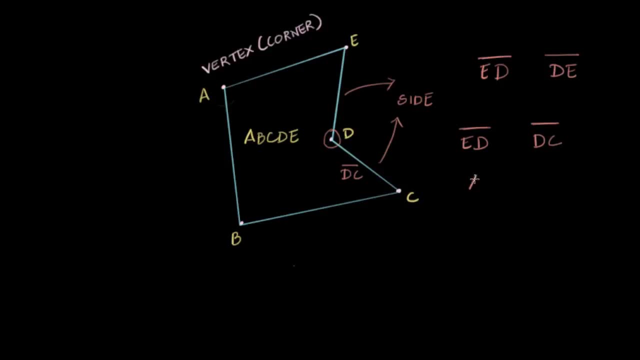 of a polygon, share, a vertex. we call them adjacent sides. Adjacent sides. Now, adjacent is just a fancy or a you know a serious sounding name for next to. So I just want to say these two sides are next to each other, So I say they are adjacent to each other. So e, d and d- c are adjacent sides. 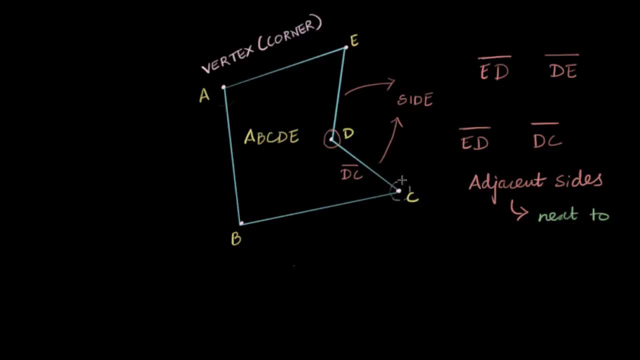 bc and dc are adjacent sides. you can always notice that because there'll be one alphabet in common between them. so if it's ed and dc, then you know that the vertex d is common. if it's dc and bc, then you can see that the vertex c is common between them. 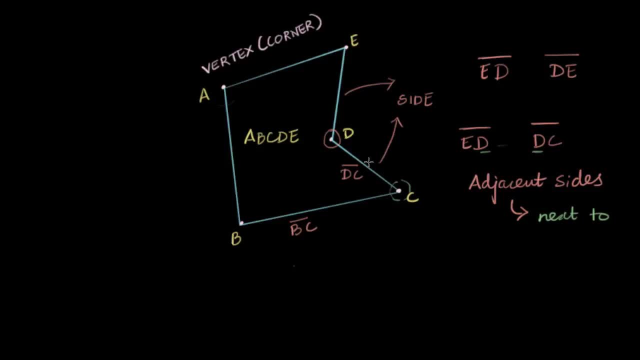 so those are called adjacent sides. now also notice that if you have two vertices- a and b- that share a side between them, so if a side connects a and b, then those two vertices are called adjacent vertices. so i'm going to write that over here, so in this case you can see a and b. 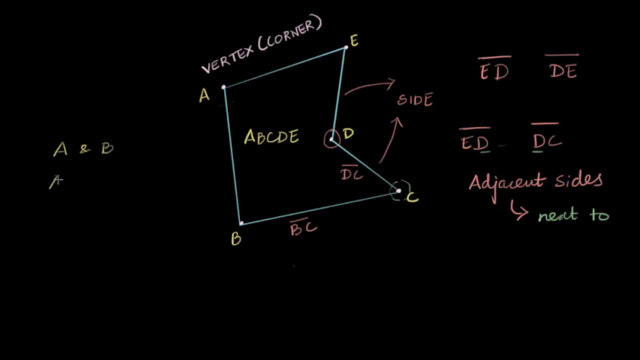 a and b are adjacent vertices, vertices. now, whenever i write vertices i can see that. you know, vertices are just a plural of vertex. i used to keep writing vertexes when i was a kid: v-e-r-t-e-x-e-s, which is not correct. we just had a mini english. 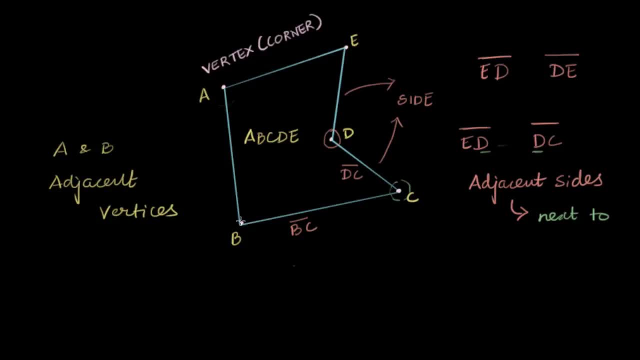 letter v-e-r-t-e-x-e-s which is not correct. we just had a mini english letter v-e-r-t-e-x-e-s and over there. so you have a- b, which are adjacent vertices. b- c are adjacent vertices, basically next to each other corners, if you want to think about it that way. but you can see that a and d are not. 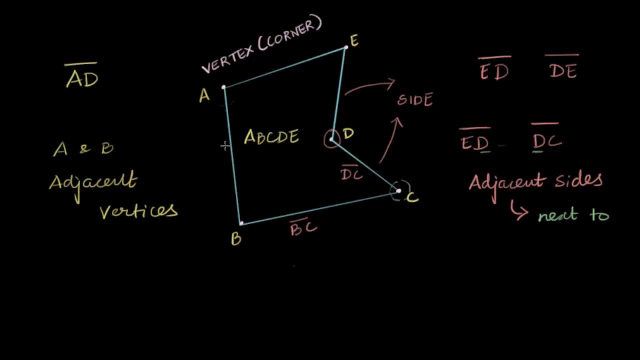 so if i write a, d and put a line like this, this is a line segment that connects a and d, but then that's not a side of this polygon. so can this be possible? yeah, it is possible. i can just draw a line segment, but that won't be a side of this polygon, that will be something else. so that's ad. 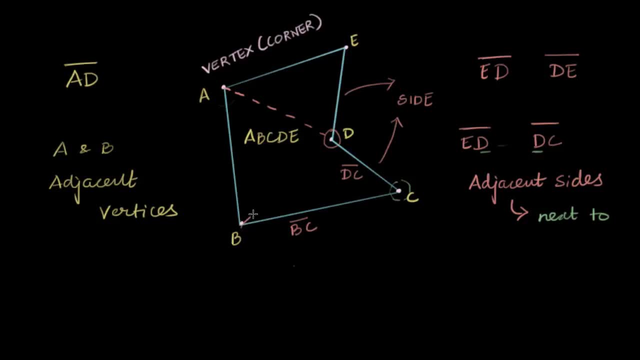 so maybe i can draw bd bdo here as a solid line and now bd again. b and d are not adjacent vertices, so whenever you connect two vertices that are not adjacent with a line, the line that you just drew now is not a side but a diagonal d-i-a-g-o. maybe i should use a different color: d-i-a-g-o-n-a-l. 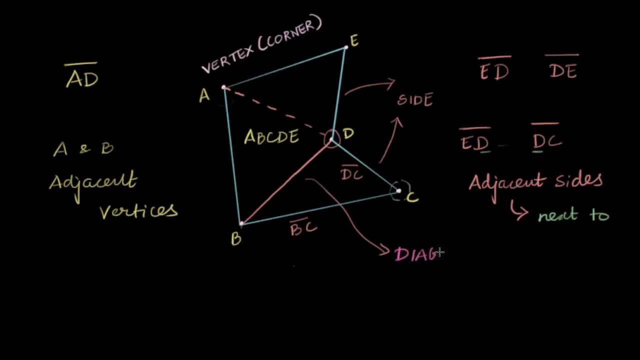 diagonal. this is the diagonal. this diagonal is basically bd because it connects the vertex b and d, which are not adjacent.